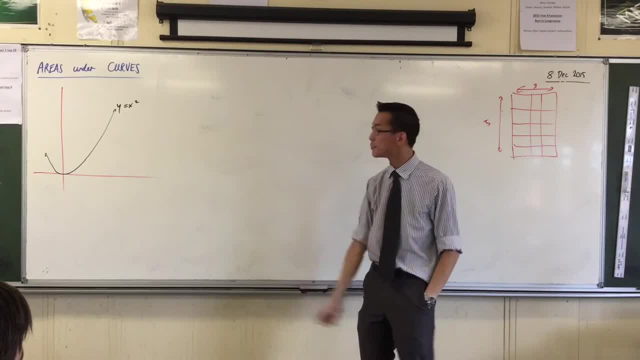 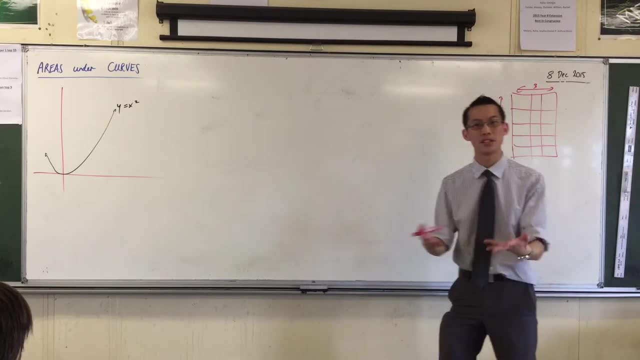 And yet, if you've got this graph, this little parabola drawn up, despite its simplicity, it sort of disguises, hides these very, very deep questions. Example: okay, We know how to find the area of rectangles. What other kinds of shapes do we know how to find the area of? 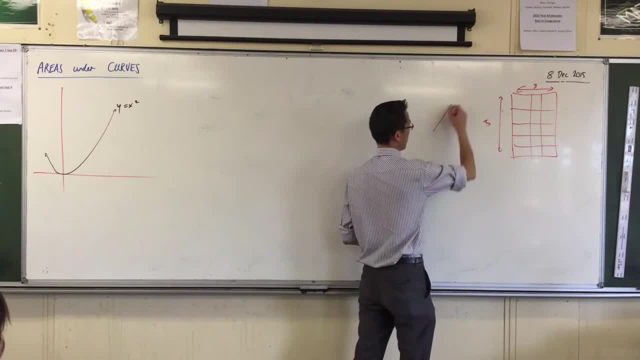 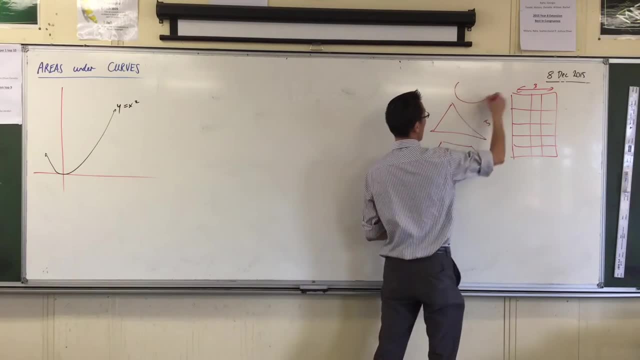 Example: Triangle, Triangle, Trapezius- Okay, we can do trapezia right. What else Circles? Circles, In fact. you can work out the area of any polygon if you like, as long as it's got straight edges, and you can work out circles. 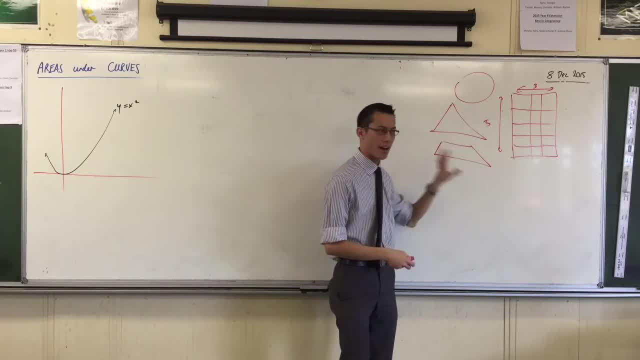 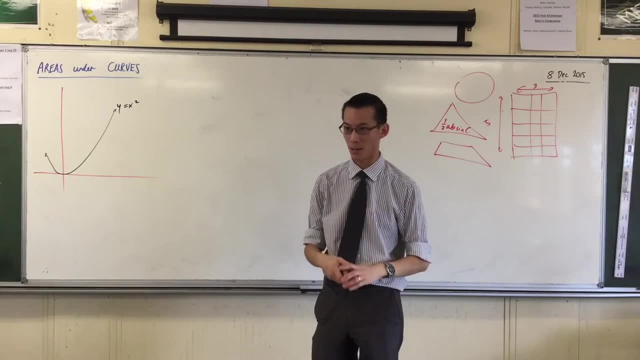 Are you happy with this idea? And we spend a long time trying to work these out and we even develop really fancy, sophisticated ways of working out some of these different areas. okay, And yet if you come to almost one of the most simple curves, 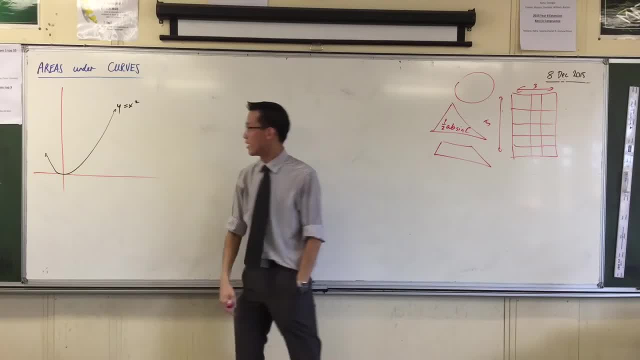 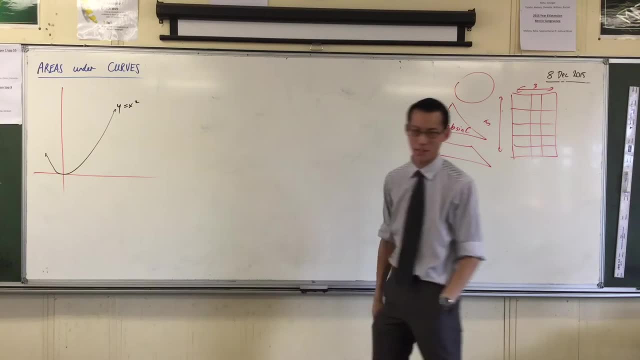 that we know how to draw right. In fact, by the definition, by the general way that people say curves, this is the simplest curve that you can draw. You can draw y equals x, but it's not curvy okay. 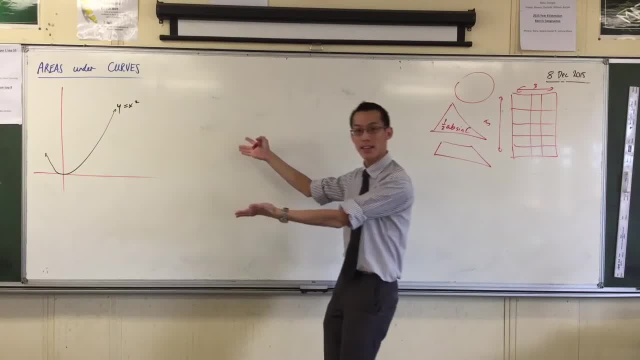 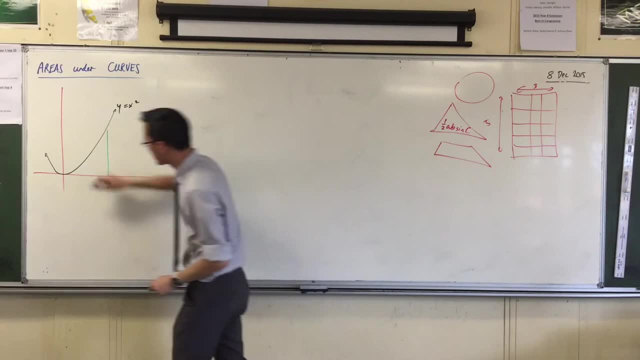 Now to try and work out the area underneath this curve. for example, let's put in some lines in here. If I put in a boundary like that and say: okay, look, here's a shape under here, What's its area? okay, 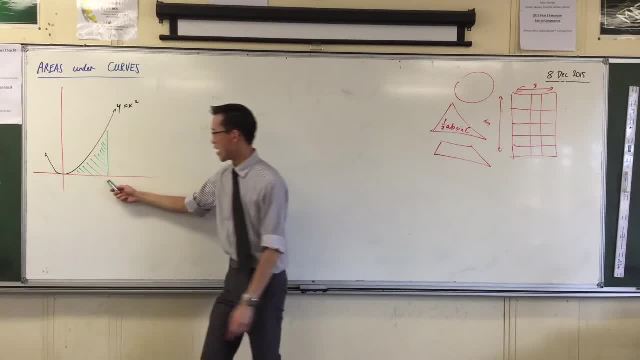 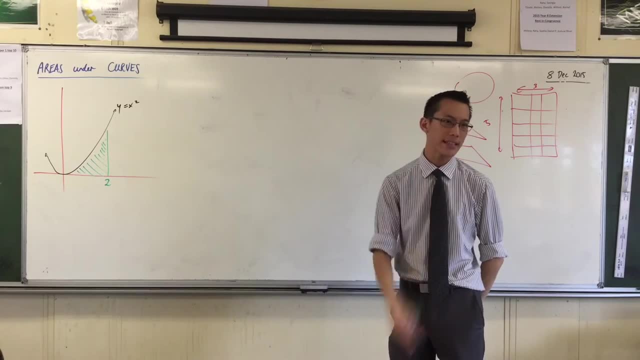 How big is that thing If you know where you start and where you end? suppose that's something, I don't know, colon two or something like that. how big is the shaded area? It's an immensely simple shape, Immensely simple. 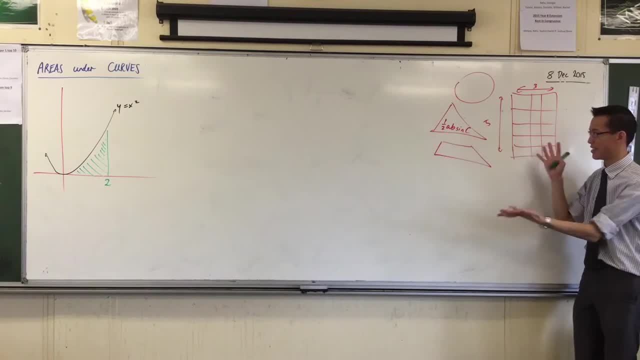 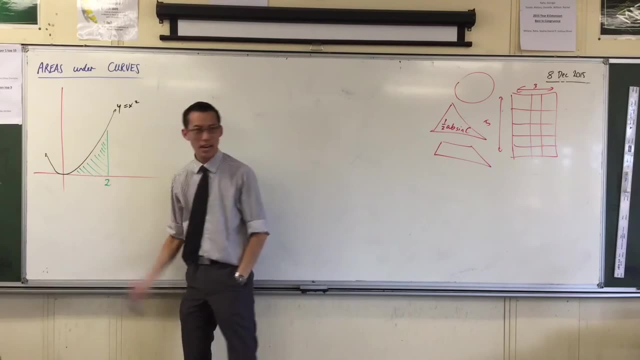 However, it defies all of this understanding we already have developed on area. There's no polygon that you can fit in there because of the nature of this shape in here that's going to be exactly equal to this area. There's not even like any combination of circles. 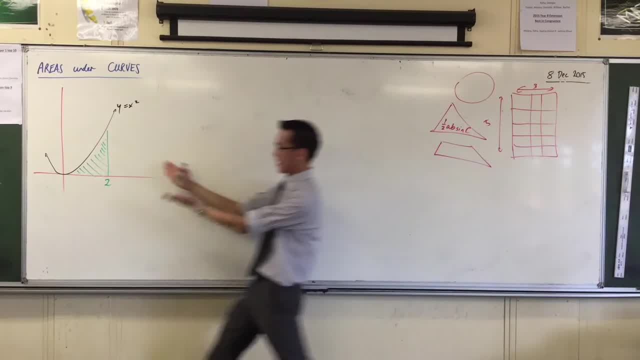 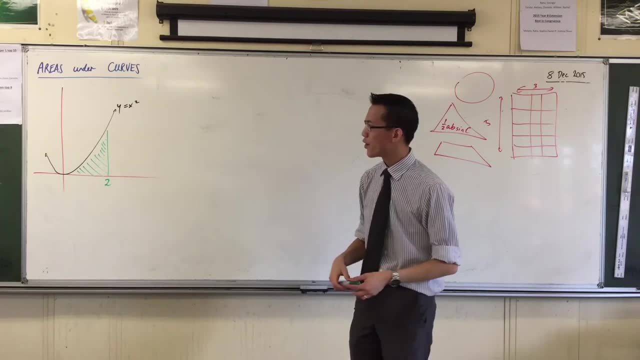 or semicircles or sectors that you can try and like, fit the curves in so that it's like nice and exact. You can't get there Such a simple question, okay. So Riemann, was this mathematician? 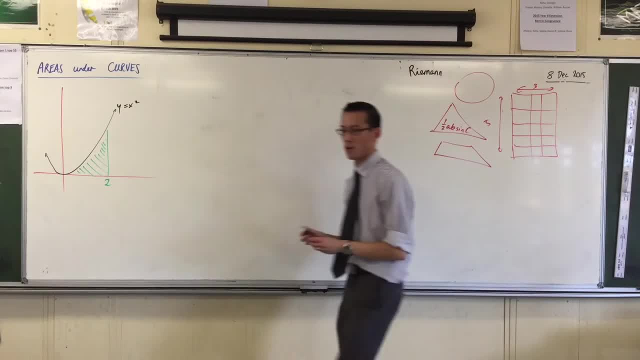 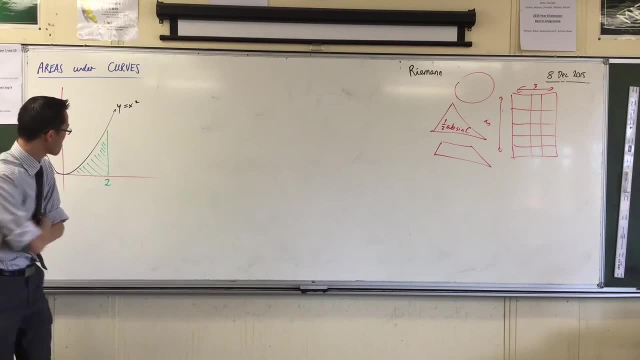 Riemann, German guy, double M worth writing his name. who saw this? this is an interesting problem. okay, We want to try and tackle this problem. So he said, look, okay, classic mathematical technique if you can't work out a problem as it is stated. 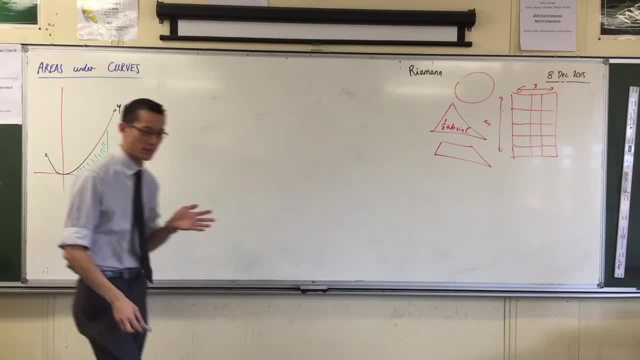 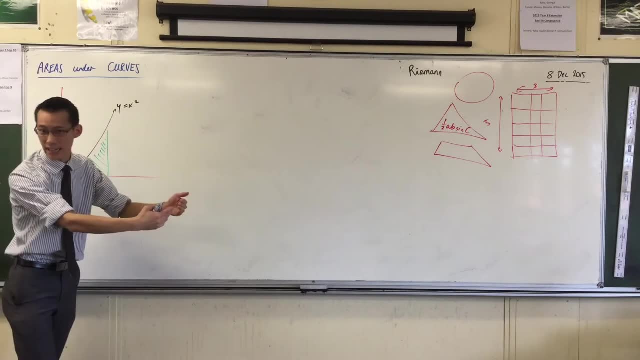 what you do is you try and simplify the problem and see if you can work out. well, can I work out an answer to a simpler version of this and maybe I can kind of like import that understanding forward? okay, So, for instance, you've got all these shapes over here. 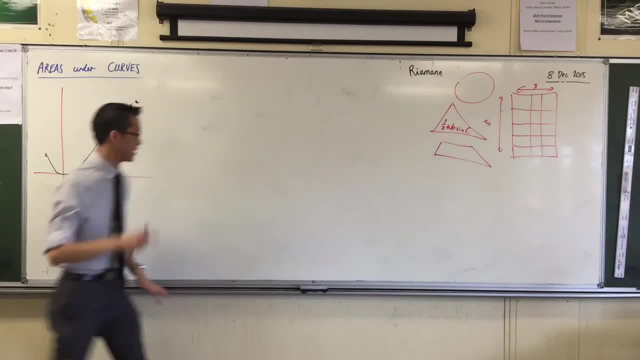 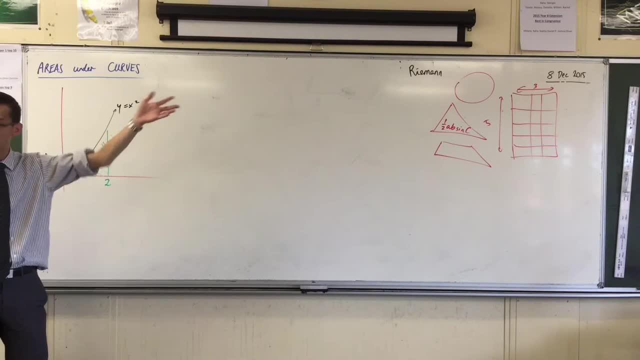 that we know how to work out the area. Riemann was really smart. He said: well, you know what I can try and approximate this area with like versions of those. So here was the first way he did it. 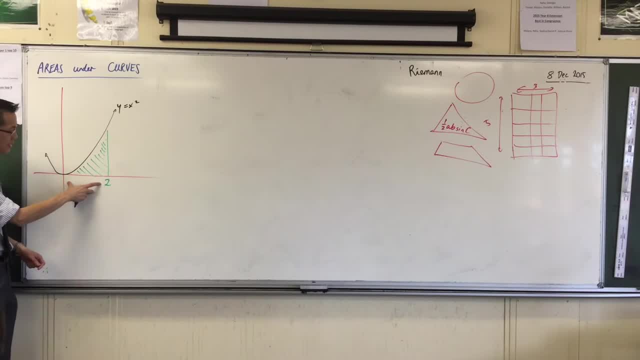 Draw some vertical lines in for me so that we can divide this interval. well, let's divide it maybe into four, for example. So if you have, okay, and then if you have these two, okay, Riemann said well, each of those. 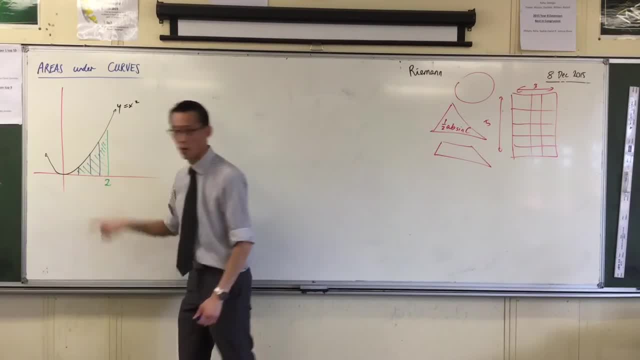 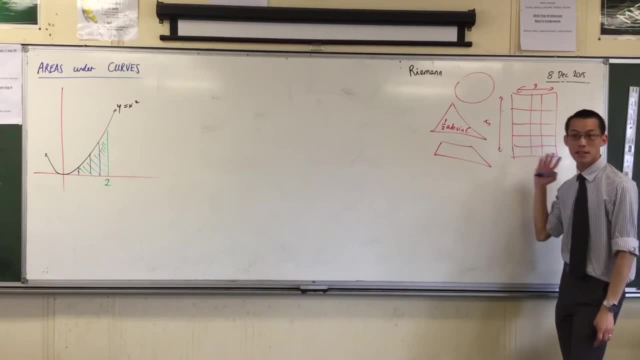 those four pieces that I've got: one, two, three, four. I still don't know what each of those is because they still have that curvy bit in them, okay, But I can approximate them with shapes that I know how to work out okay. 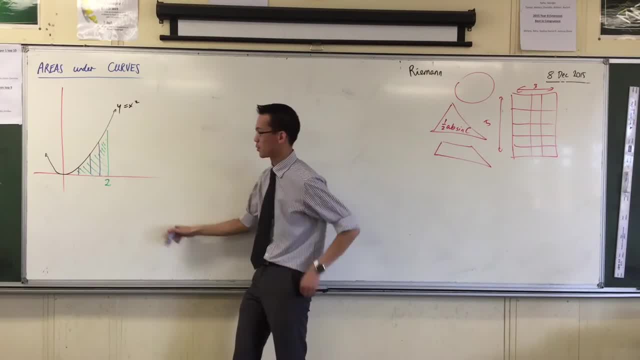 So the first way he did this- and we're going to copy this over as well- he said: look, I'm going to draw some rectangles in here, I'm going to draw some rectangles. For instance, I can draw a rectangle here. 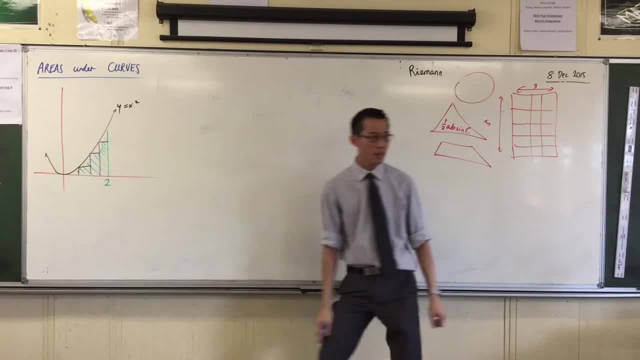 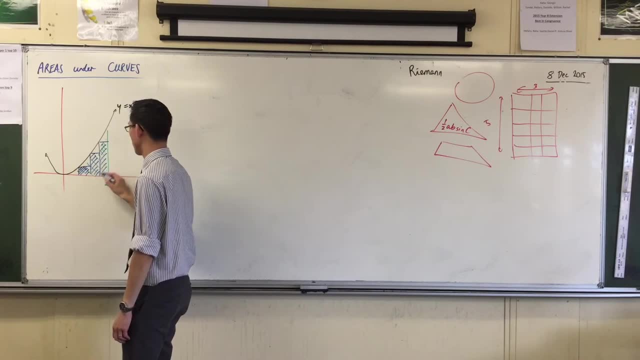 here and here. okay, Now, if I shade these in like, so there is actually, even though I've only drawn three rectangles in, there's actually a fourth, one right. Fourth one here. it just doesn't have any height. 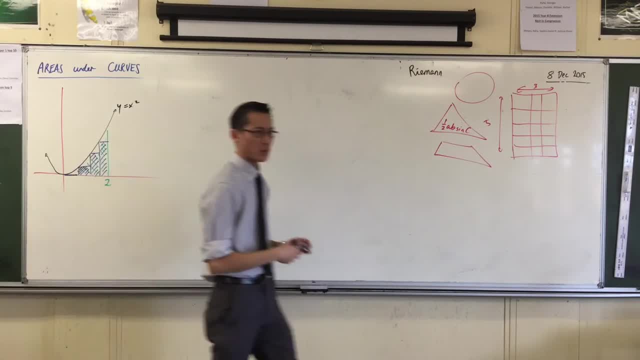 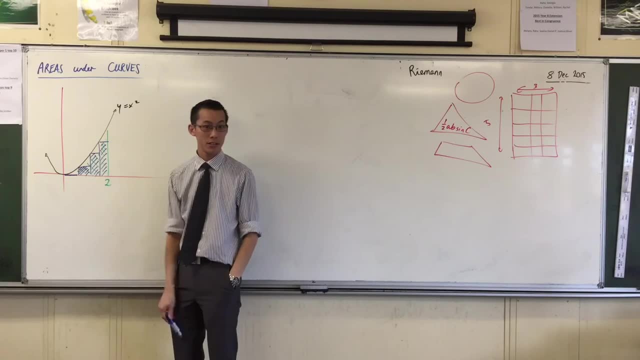 because I'm on the ground there, These four rectangles, the area that I'm after, the green area, the curvy area, it clearly is going to be greater than this area. Do you agree with that? It's just above. it's always above right. 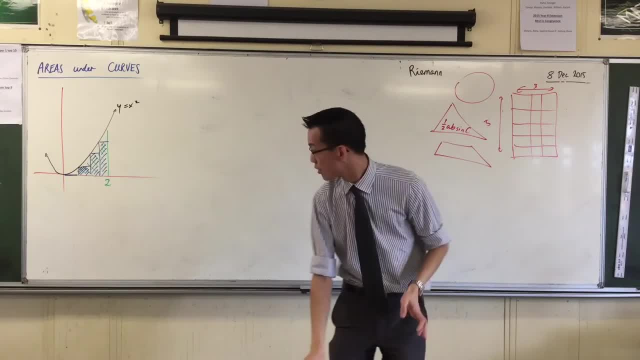 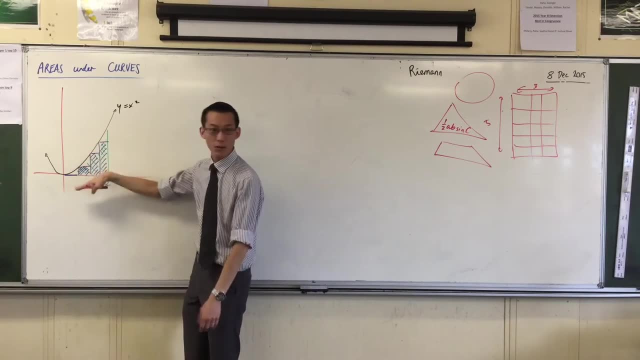 So it's like I'm missing these little gaps. okay, So that'll get close. But I can be even smarter and I can say: see these same subdivisions that gave us four. I've got rectangles underneath the curve. I can also put some rectangles in above the curve, like this: 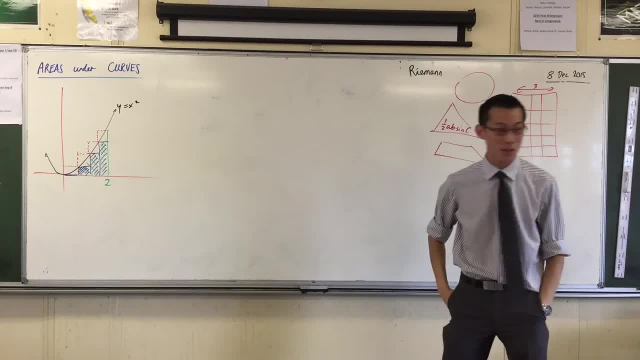 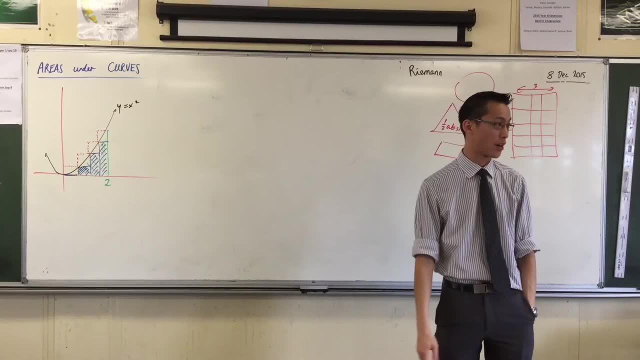 Now these are. I'm not going to colour them in because it will make my diagram too busy. If you've got enough colours, you probably can. But the areas of those four red dotted rectangles. okay, can you see? they're always above the curve. 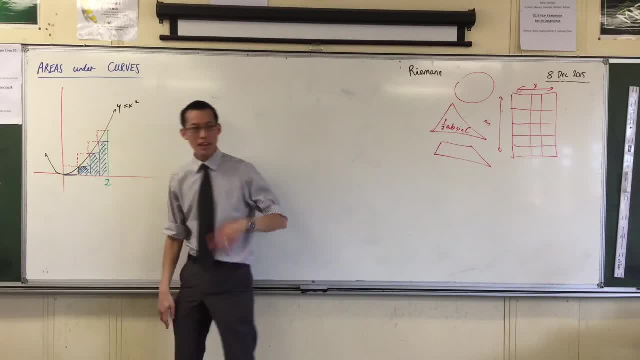 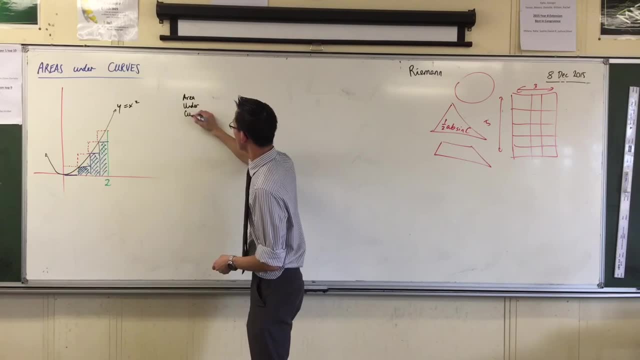 Always above, always above, Always above. So the actual area I want- right, Let me write it like this- Area under curve: okay, It's going to be less than the red dotted area And it's going to be more than. 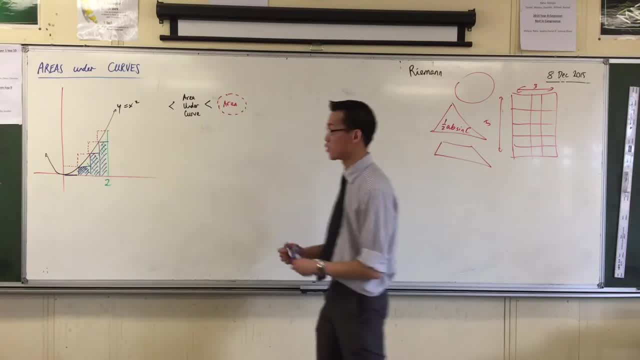 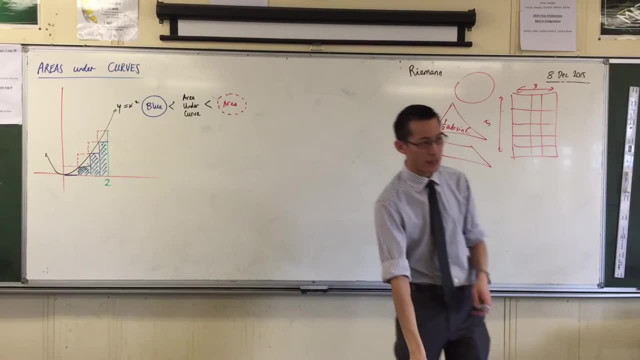 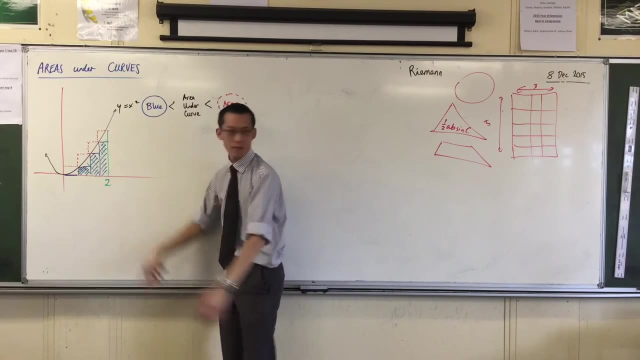 well, I call it the blue shaded area, those blue rectangles, okay. So Riemann said: hey, this is really good because, even though I don't have it exact, I can pin down this area within some actual numbers, because, well, they're rectangles. 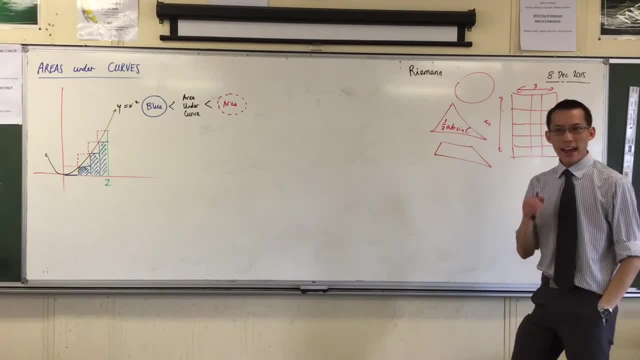 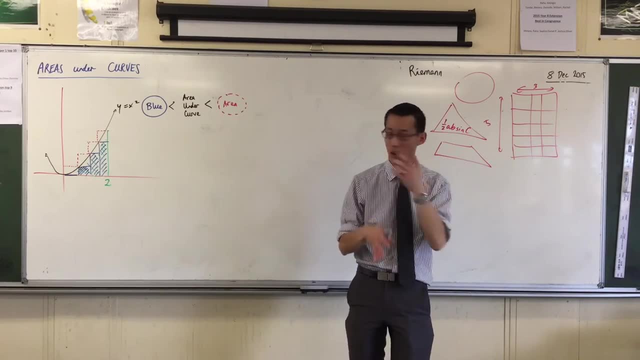 I can deal with rectangles, okay. Now here is a crucial step where we're going to differ now from where, say, an engineer, or even, to some extent, a scientist, would stop, If I can know that the area is between these two values, right? 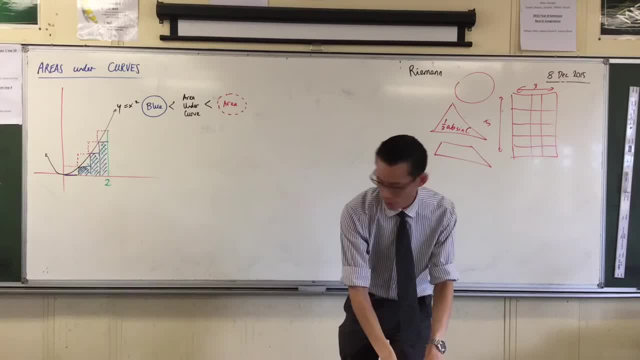 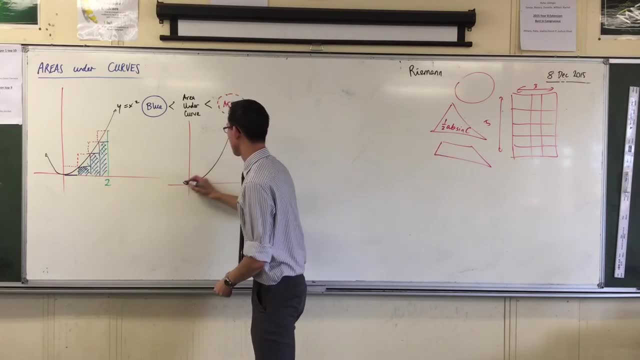 Draw a new parabola over here, next to this right, Draw a new parabola, the same one. y equals x squared, If I know it's between these two values. all I need to do is to get these. oops, that should have said area. 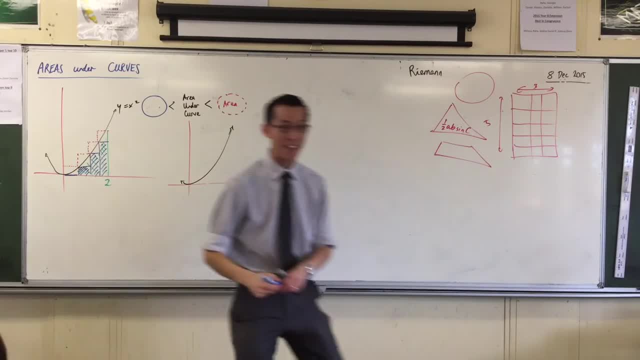 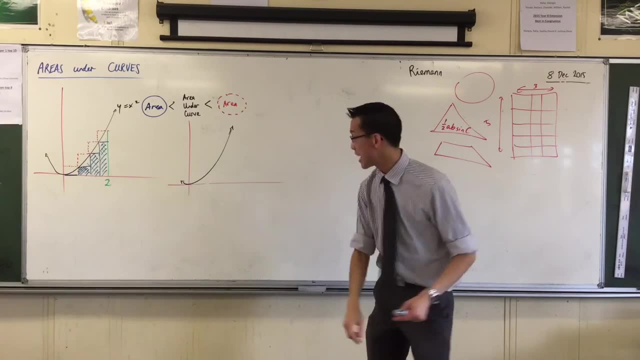 is to get these two areas, the blue one and the red one, to get them really really close together. okay, To get the blue rectangles underneath and the rectangles, the red rectangles, above, to get those values very, very close, okay. 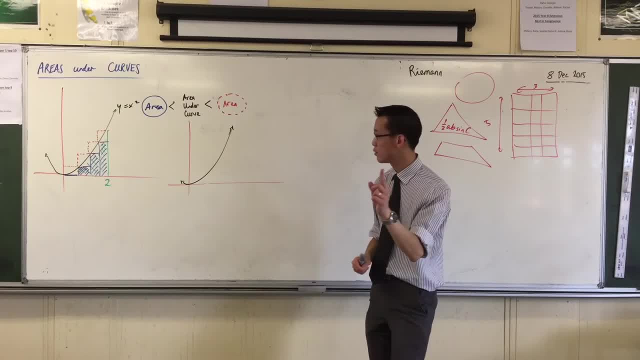 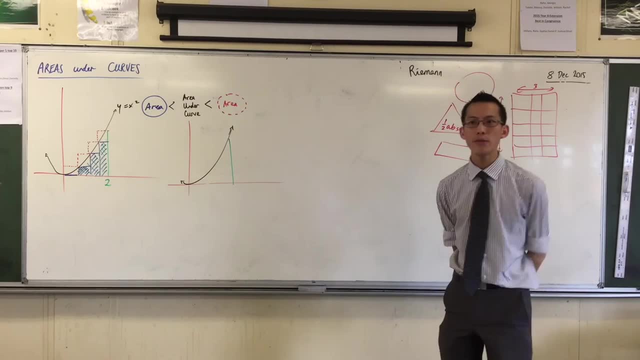 Now Riemann said: okay, I know exactly how to do this, right. Instead of dividing this area up, for instance, into four slices, what if we divided it into more right, Like say, we divide it up into four? 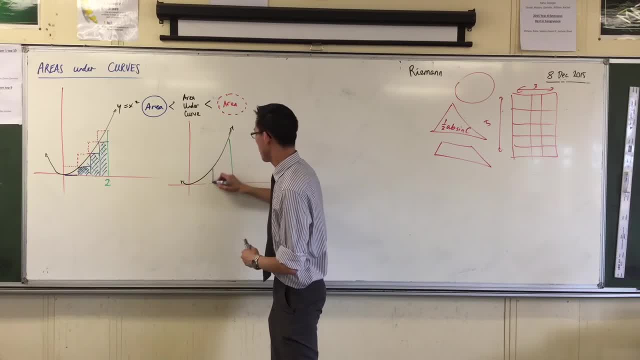 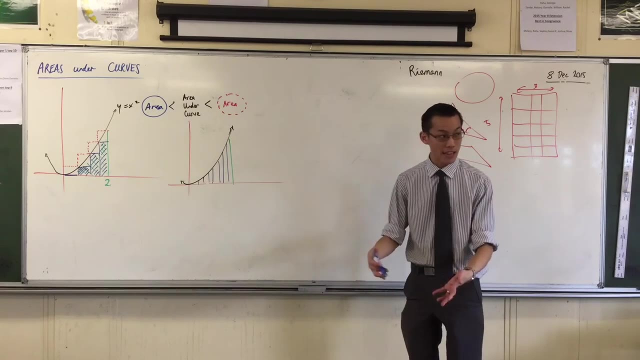 Let's divide it up, let's double it. So there's my four. And now, if I halve every one of those little intervals there, one, two, three, four- okay. Now when I draw my rectangles, okay, And in fact it's actually important that we draw the rectangles. 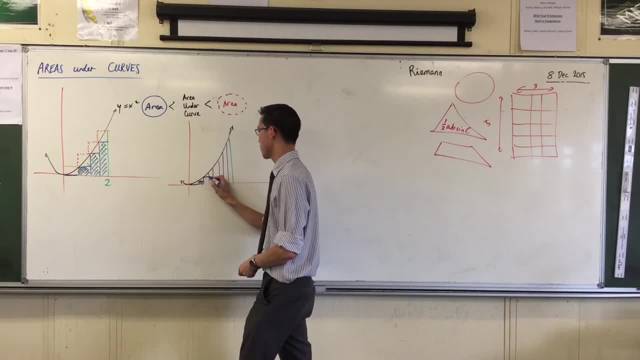 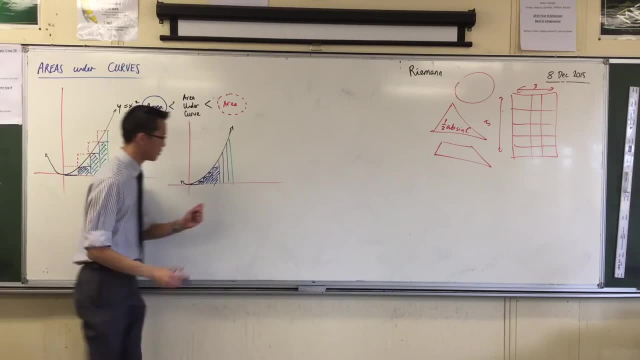 You've got the first one there, the second one there, and so on. What I want you to pay very close attention to is have a look at those gaps, The difference between the actual area that I want, the curved area, and all of these rectangles that I'm now adding into this diagram. 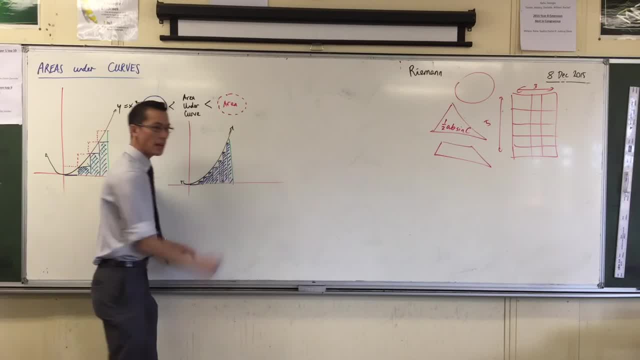 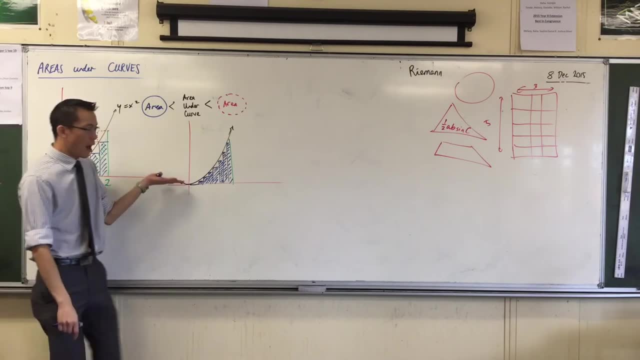 Do you see that these gaps have gotten smaller? Do you notice that? Okay, These gaps here are pretty huge. You can see them very obviously. I have more gaps, but they're all smaller. They're all little little triangles, And in exactly the same way. 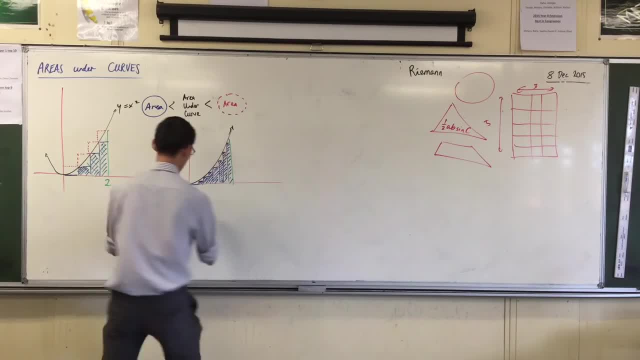 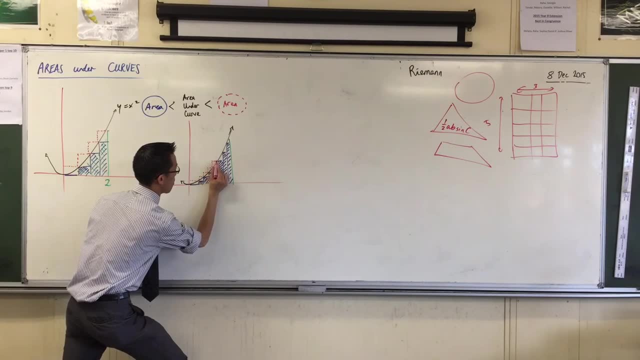 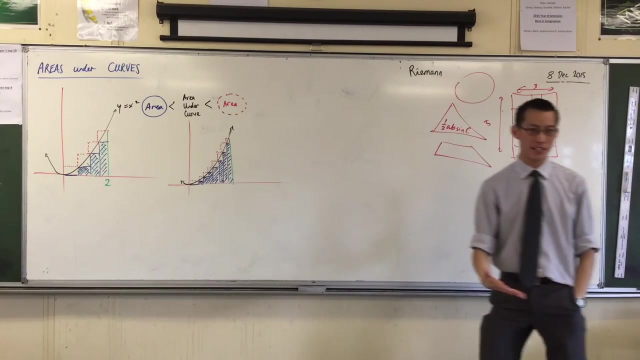 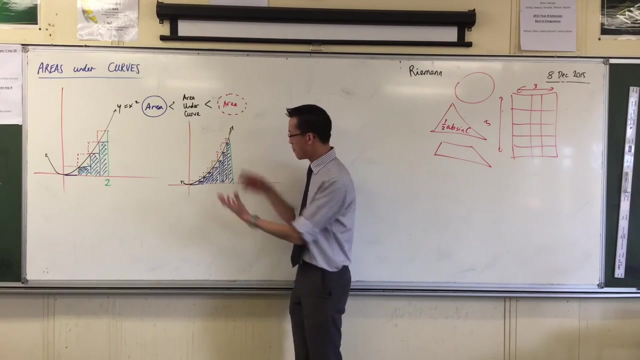 when I put in the red rectangles that go over the top of these guys like. so the blue area underestimates the area under the curve And the red area overestimates the area under the curve, But the overestimation and the underestimation are now smaller, right. 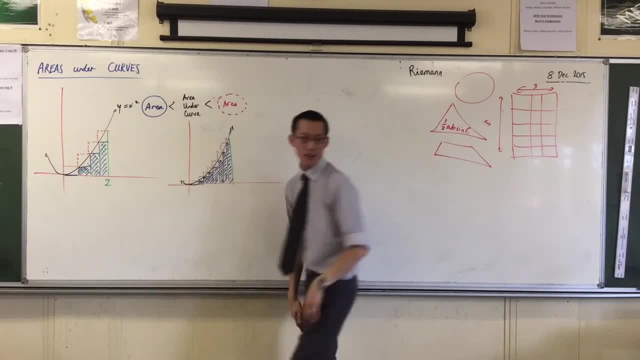 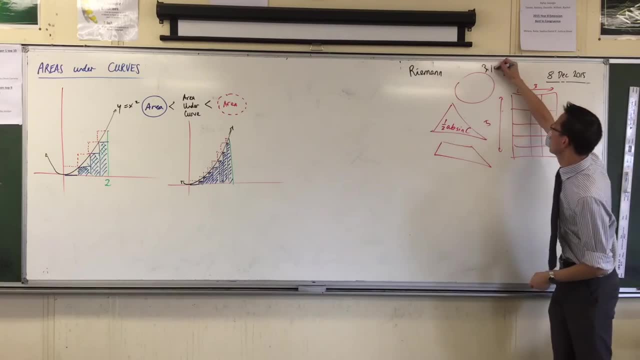 So these two numbers are going to get closer to each other. Now an engineer would say: look, I just need this to be close enough. Close enough, Like people say. oh yeah, you know, I know. 50 million, billion, whatever decimals or plus. 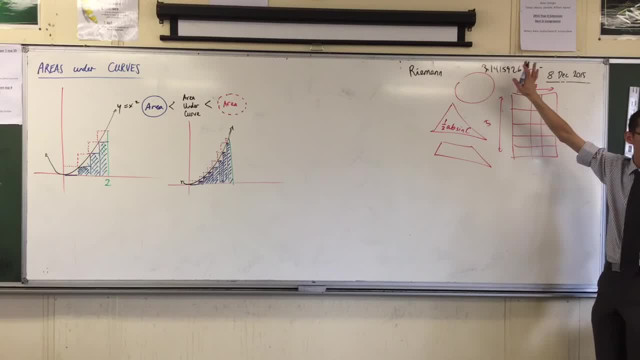 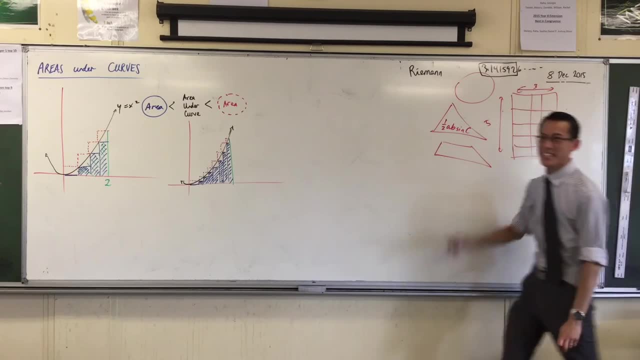 Decimals or pi right Engineers will only ever use about six, About six right One, two, three, four, five, six. At that point there, that's insane accuracy Enough to do any like building or bridge you're dealing with. 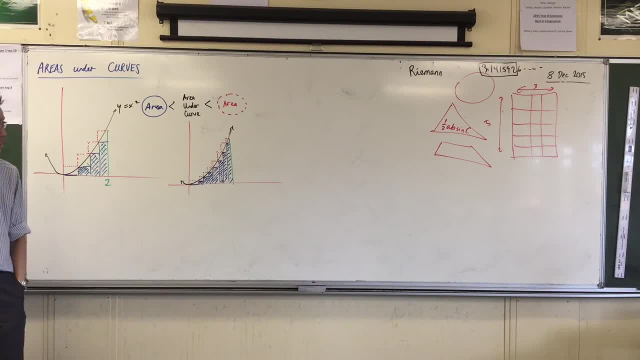 That's just fine. if you want to make a circle, You don't have to have any circles in your design. All an engineer would need to say is: okay, so long as I can get close enough, so long as I can get these numbers close enough together. 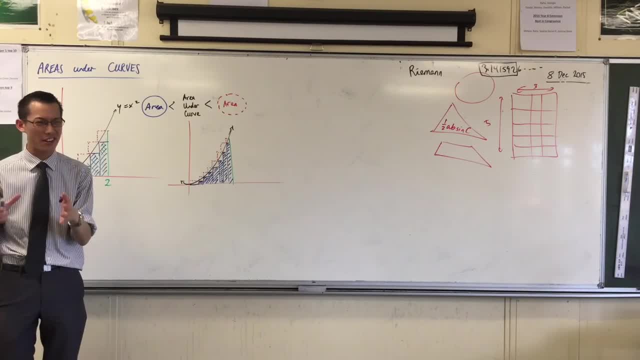 I'm happy, right, I've got something that's accurate enough for me to work with. Okay, But in this classroom we are not engineers or scientists, We are mathematicians, right, And mathematicians are never satisfied with close enough. 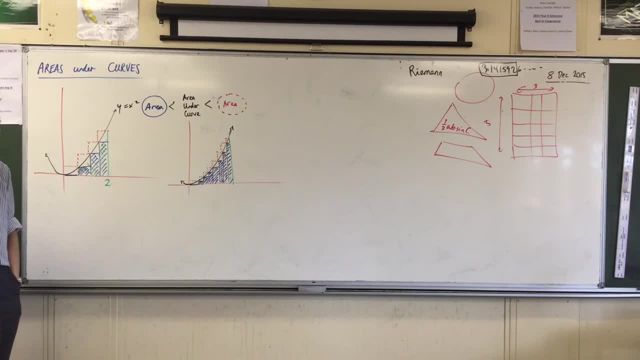 We say: can we get this exactly Okay. So in order to do that, we need a bit of language to describe what's going on.